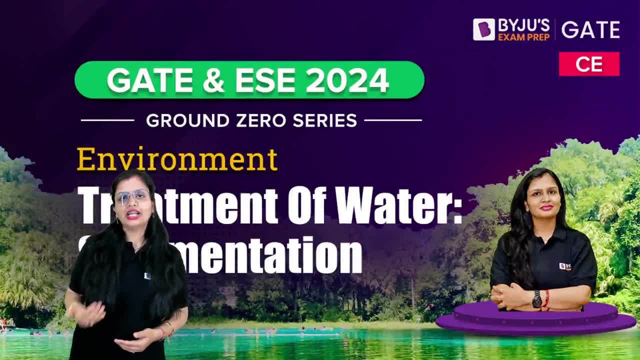 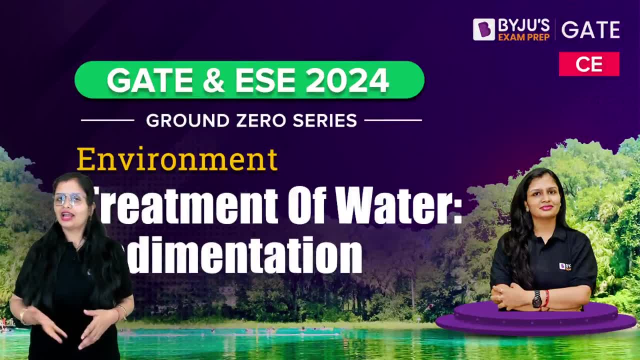 is those suspended particles who have weight, who have specific gravity greater than that of water. A water is basically well, it can be wastewater or it can be raw. water will settle down under the action of its own weight. So, generally, when you talk about basic 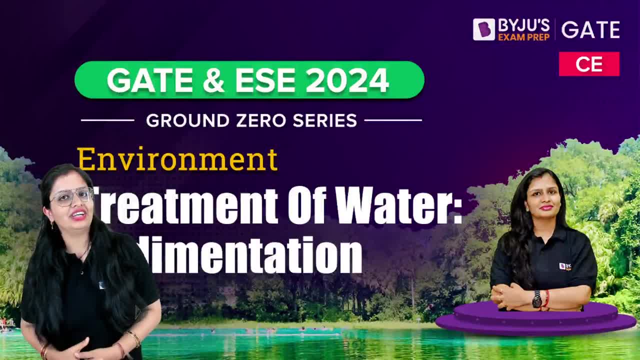 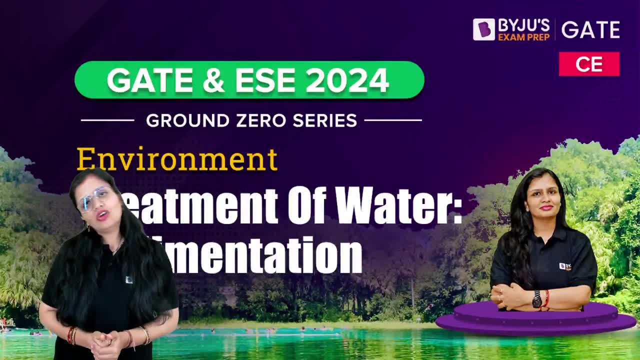 study you will be talking about sedimentation. So in this video I am going to talk about sedimentation. sedimentation, we have the hero: specific gravity. and specific gravity stands for what? Weight of solids of given volume upon weight of fluid of equal volumes. Now comes the question that when 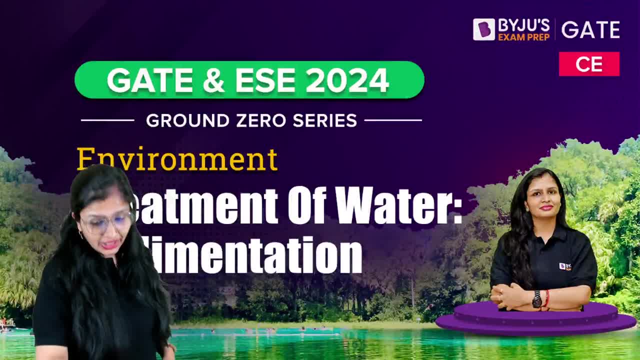 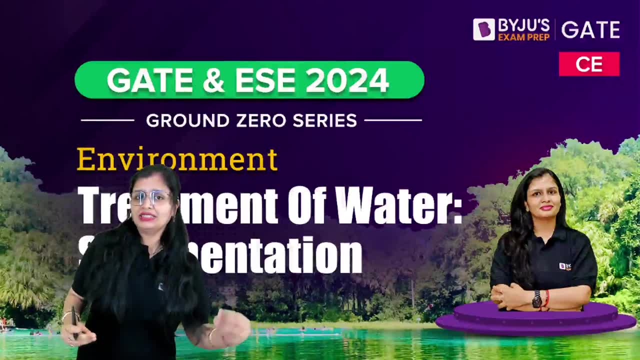 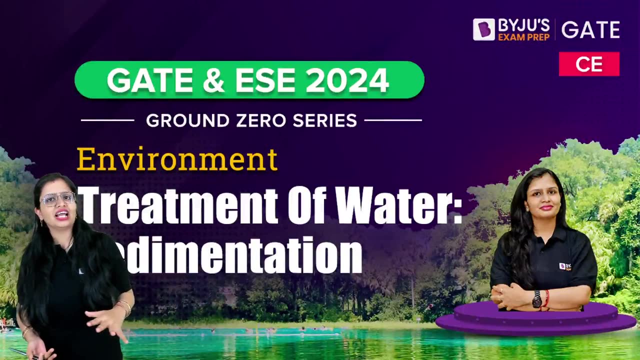 I am talking about sedimentation and I am telling you that the hero of this is specific gravity. so the next question which comes into action is: do the specific gravity varies for different types of solids? Yes, If you talk about organic solids, the specific gravity is generally in the range of 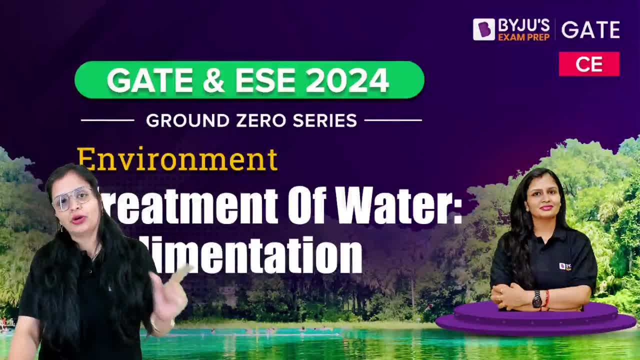 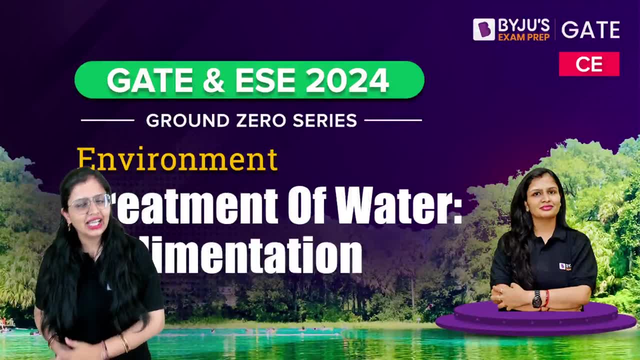 1 to 2.. If not mentioned anything, we take it as 1.2.. Specific gravity of inorganic solids generally varies from 2.6 to 2.9.. If not mentioned, we take it as 2.65.. Now coming up further, let us talk. 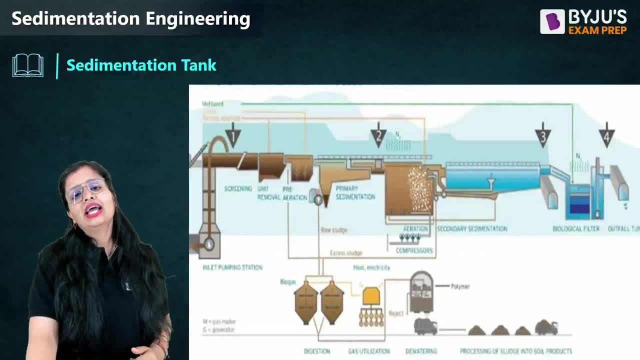 about it in further, detailing that sedimentation, this process, where the help of which the removal of fine suspended solids, those solids which are not removed in screening, are being removed in the sedimentation tank. okay, because these are finer in nature and we know screening does the removal of heavier and last suspended solids. So the 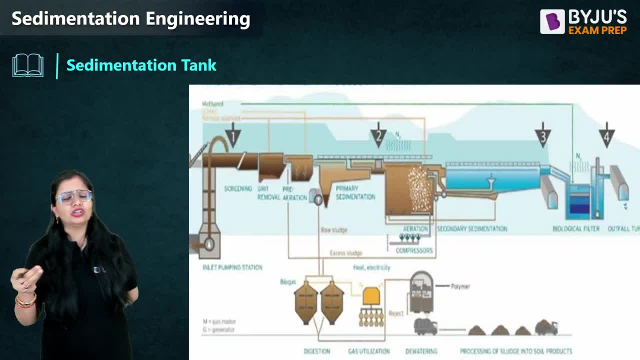 question comes into picture is when you are talking about the removal of last suspended solids, which was done in screening. now the fine suspended solids will be removed in sedimentation tank. So the question comes if we have one sedimentation tank or two sedimentation tanks. 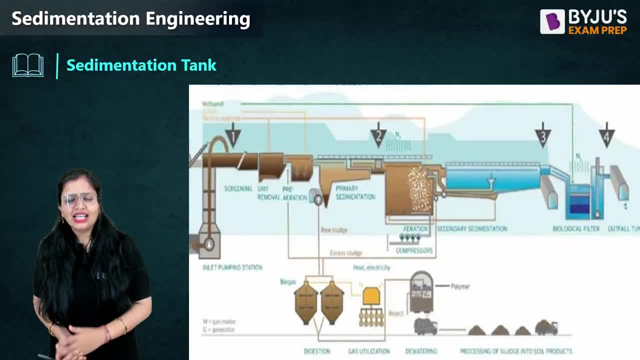 so it varies, Varies, ma what do you mean? like if you talk regarding downro water treatment, that what object is supplied to your home from the source, There we go for only one sedimentation tank. but if you talk about wastewater treatment, where the water from your homes after being used, 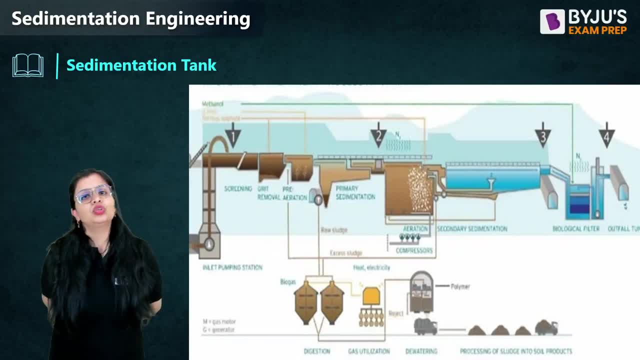 is to be disposed. So for that we have two sedimentations tanks, and for sedimentation tanks we have to also take about that product to be desposed. sedimentation tank one is primary sedimentation tank and the other one is secondary sedimentation. 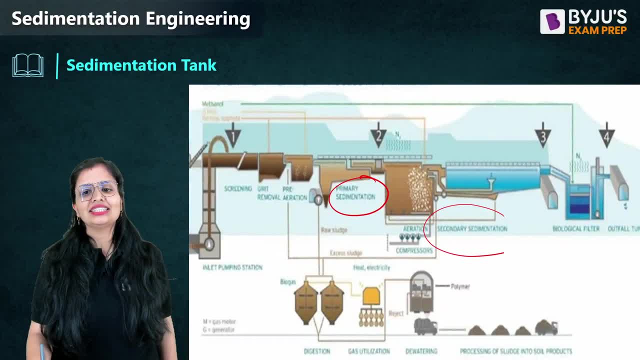 tank, so you guys can see it here also: primary sedimentation tank and secondary sedimentation tank. so basically, the purpose is you want the removal of fine suspended solids now comes into action. that do. we have a well-defined, a single sort of sedimentation tank or they vary according. 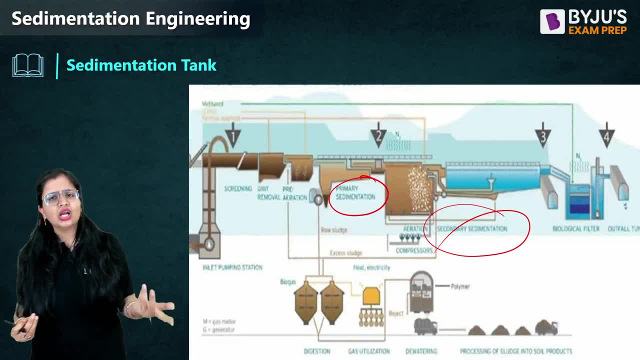 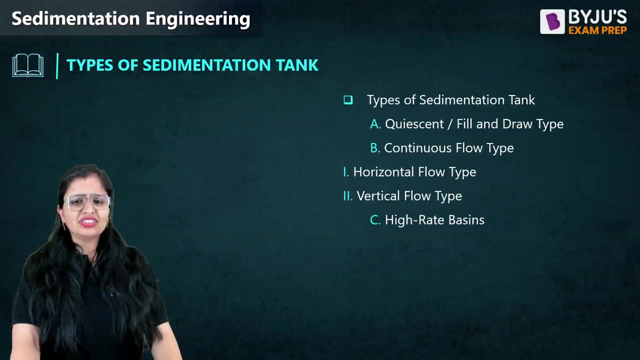 to the shapes, or they vary according to the functioning. what is it? so? let's talk about it now when you talk about the various types of sedimentation tank broader, since we started to. but actually there are three types of sedimentation tank. first is quiescent type tank, which you call. 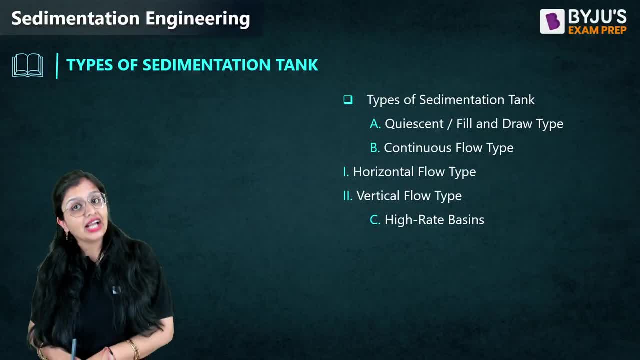 it a fixed type tank also and you call it as fill and draw type tank. secondly is continuous flow type tank. in this you have horizontal flow type tank, vertical flow type tank and the last one is high rate paces. if you talk about the ones which we focus predominantly is type a and 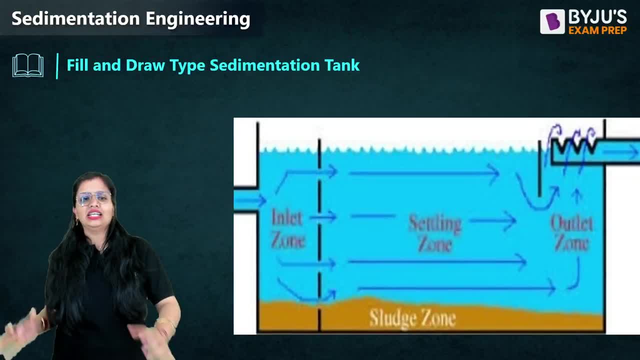 b, type B, Now coming up further. so you can see, let's move towards fill and draw type sedimentation tank first, As the name suggests, you fill the water in the tank, the water which is to be treated. Okay, fill the water Here you are bringing the water to rest. That means turbulence. 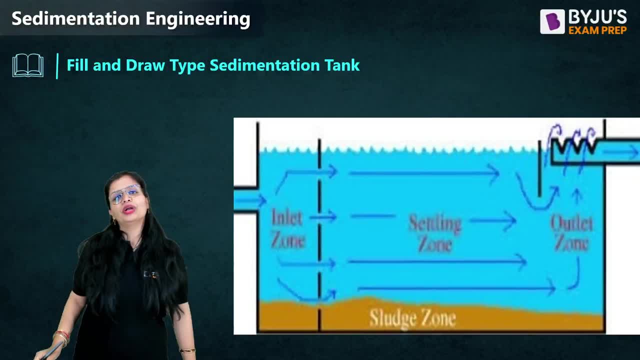 is zero. There is no haphazard movement of water. So when it comes to rest, the particles will eventually settle down. After that you will take out that water. That means you will draw the water. So you can see here, this inlet zone is there. From here the water will go into the settling. 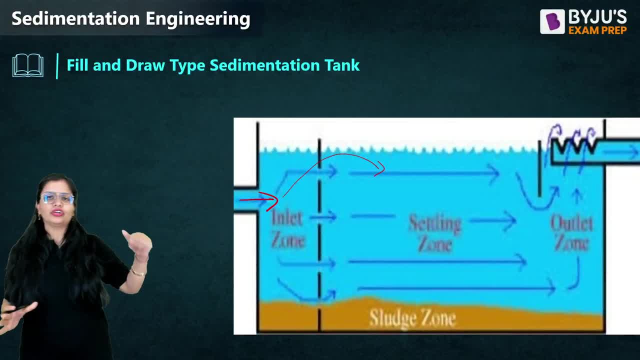 zone, Inlet zone. let us suppose the water from screening or water from aeration will go into the inlet zone. From the inlet zone it will go into the settling zone where specific gravity will come into action because you have made the turbulence zero. The water is at rest, So the particles 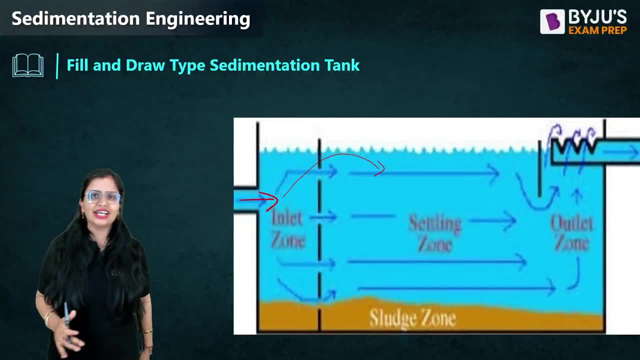 particles who have a higher specific gravity will eventually settle down. So here what you will see: settling will take place and that water will again go to the outlet. okay, So you have settling zone, the particles, the solids, which you have settled down along with the combination of water. they 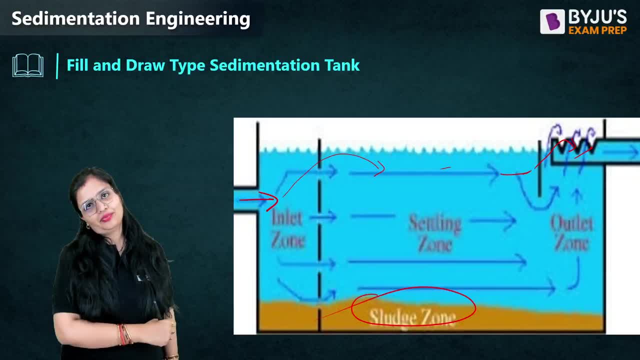 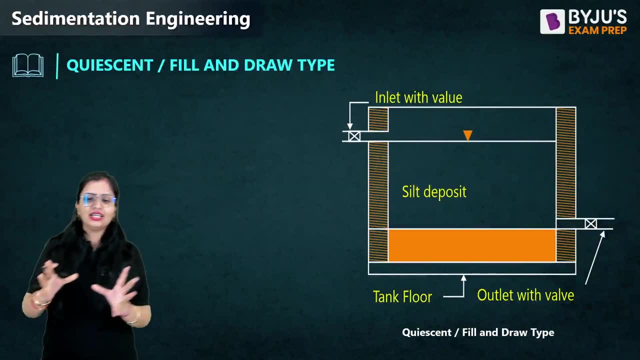 will form sludge. So that's the reason you have a sludge zone. okay, So you have four zones If we go in further detail, so you can see it here. that inlet is there, silts deposit tank floor is there. 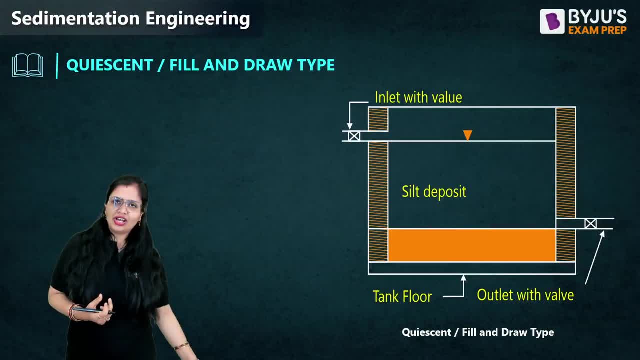 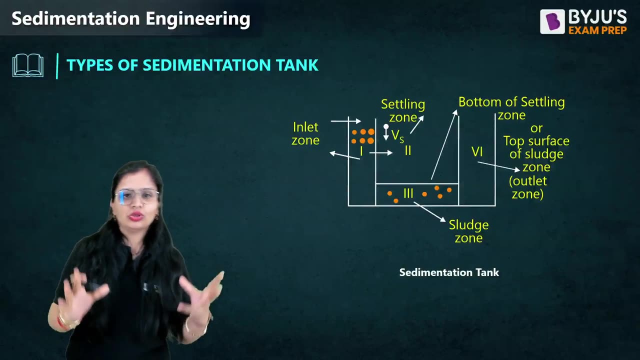 and you have valve. Now why does this? valve is provided for the proper regulation so that the suspended solids get settled down and we can eventually get higher efficiency. So valves is provided for that. Now, if you want to see, as I told you about the zones, so inlet zone. 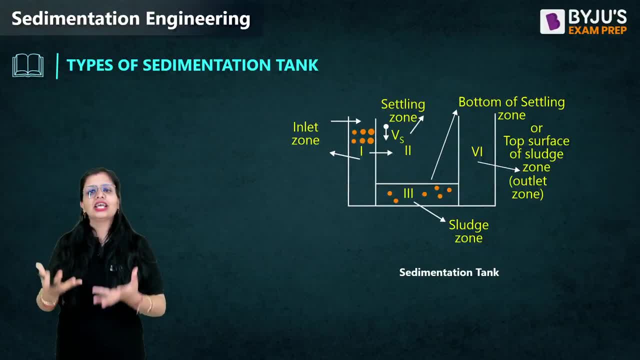 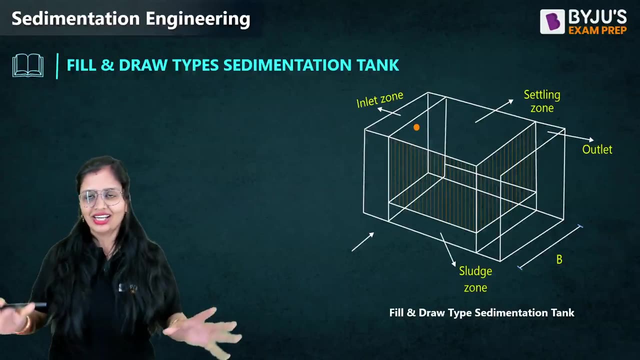 settling zone where the settlement of particles will take place. eventually, it will lead to the formation of sludge. So, as I told you guys, after that we have what, we have the, we have the outlet zones. So this will be four. Okay, Now coming up next, if you want to see the 3D face of it, see, I don't want that you are seeing. 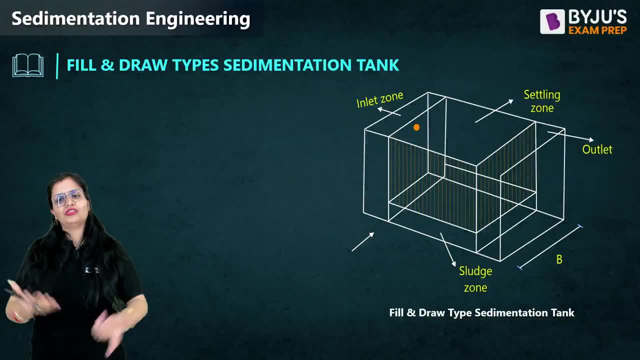 the plan or you are seeing the section. you can see it in every manner. So if you want to see the 3D view of it, you can go through this. the inlet zone, settling zone, sludge zone, outlet And, specifically, as you already know, that if you talk about wastewater, the sludge which is 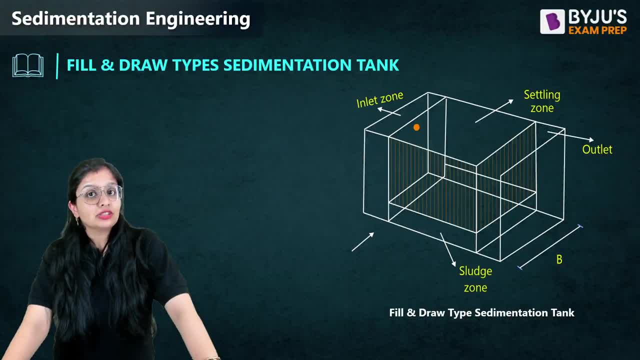 there is the waste water. So if you talk about waste water, the sludge which is there, is the there. you cannot directly dispose it, which you call it as primary sludge. So we go for further treatment in sludge, digestion tank Sludge, if it is okay and it can be disposed without any adverse. 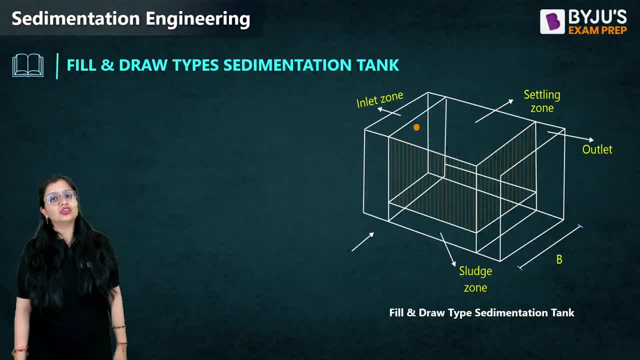 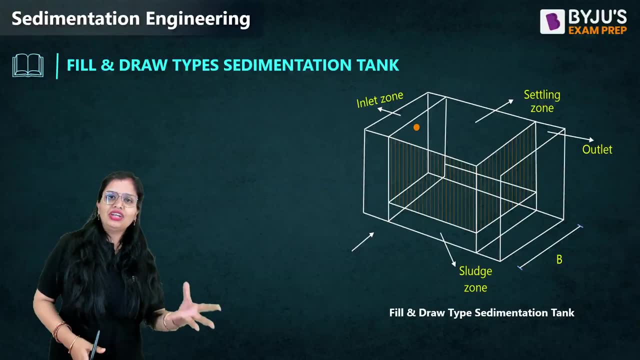 effects, it's okay, But if it is not, you have to do its further treatment before it's disposed. Okay Now, talking about fill and draw type tank, you should know that we design it for maximum daily demand. The detention time varies, But here you basically have three tanks. Two is 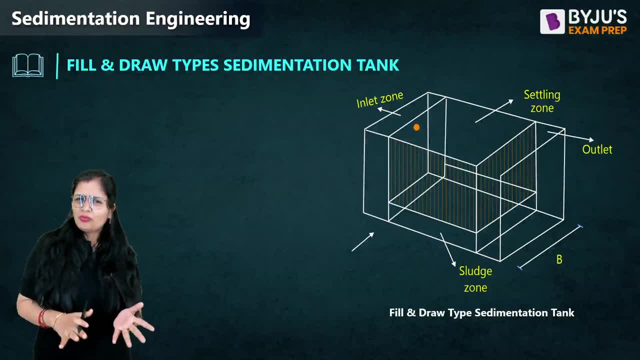 operational and one is standby. Two operational, one standby. Why? Because, see, generally we take it as 24 hours of detention time and the period of cleaning varies from 6 to 12 hours. Okay, So like when one is being functioning, when one is being cleaning, other has to be functioning. So 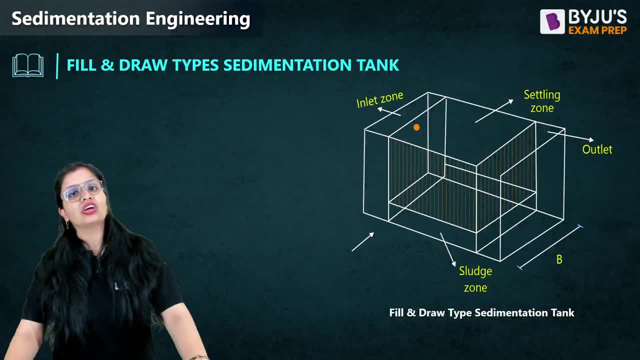 we have to have two In between. if somewhat operational troubles and all is there, maintenance for that tank is gone. So that is the reason we should have one standby. So minimum we require three tanks: two operational, one standby. Cuisine type tank is designed for maximum daily demand. Okay, And 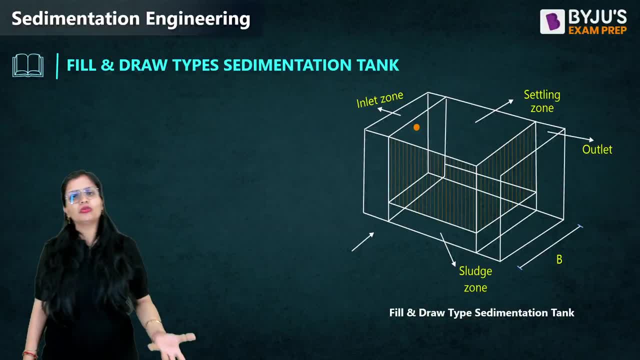 you can do manual cleaning of the sludge, because sludge has to be cleaned from time to time, Otherwise accumulation of sludge will take place. So we will get: if you don't clean it, accumulation of sludge will take place, as I said, And eventually the 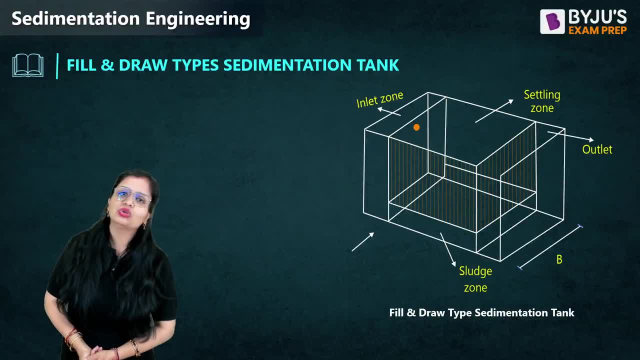 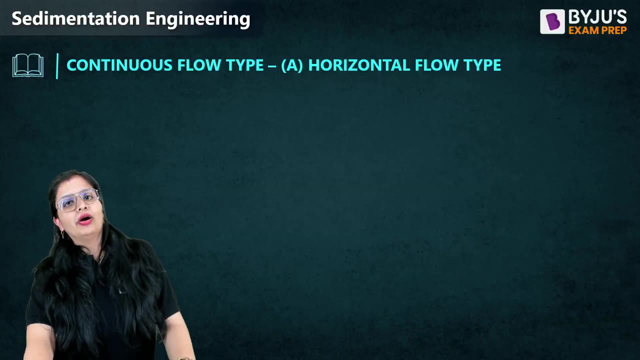 the amount or the place which is available for settling zone will reduce. Okay, So fill and draw type. question type: fix type, because turbulence is zero. Filling the water settlement, drawing the water: Okay, So this is the thing which you should know Now, talking about continuous flow type. 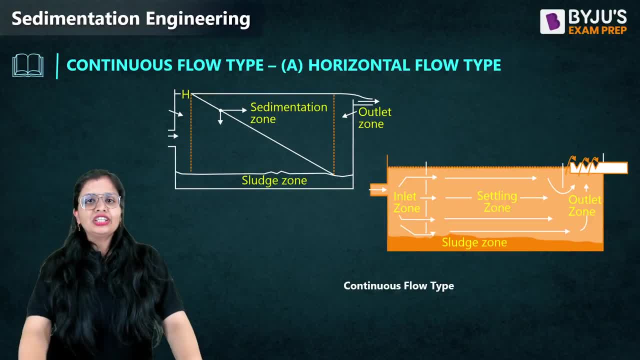 tank. here you have horizontal flow type tank which, if you see from the top, you will see it as rectangular in nature. So you have inlet zone, you have the settling zone, you have the sludge zone and outlet zone. So now, what is the difference between fix type tank and continuous flow type tank? 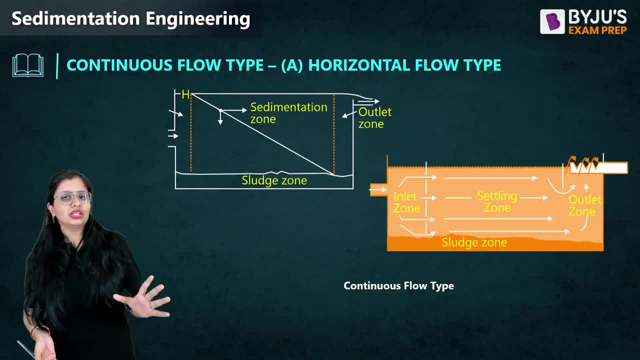 When you talk about fix type tank, actually what is happening in this case? here the movement is taking place. That means the turbulence is not zero. movement of water is taking place. Obviously, the turbulence is not there at a very high speed. that half. 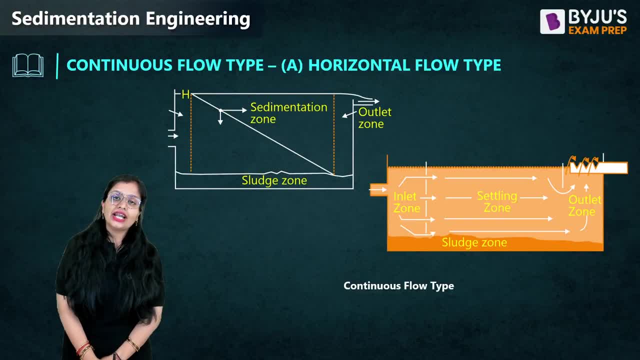 of that man of water is taking place, So that means the turbulence is not there at a very high speed, that half of that water is flowing, but stay, it is not at rest. That means what that is flowing in this case. So you will be like when the water was at rest. 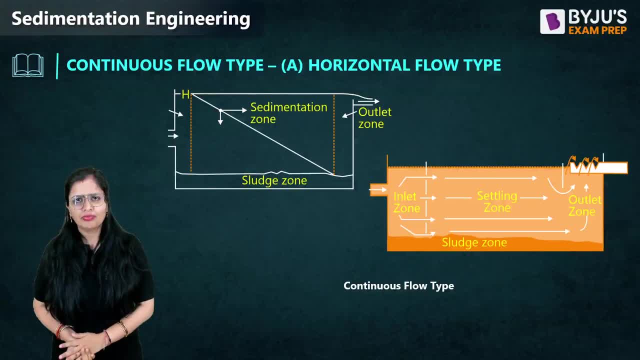 obviously what have been suspended solids will settle, what them both we. the water is moving, How will the suspended solids second? So let me tell you basically, when you divide it into two zones- settling zone and sludge zone- there are two projections which we take. let me tell you assumptions. 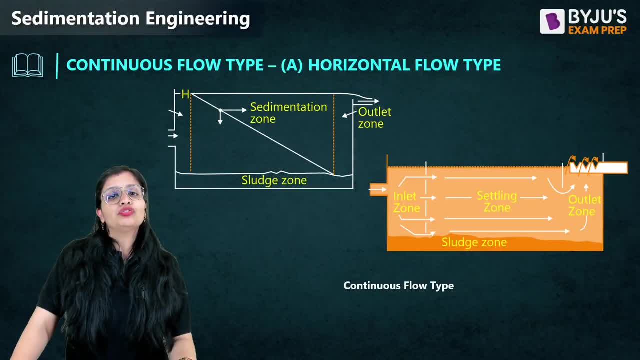 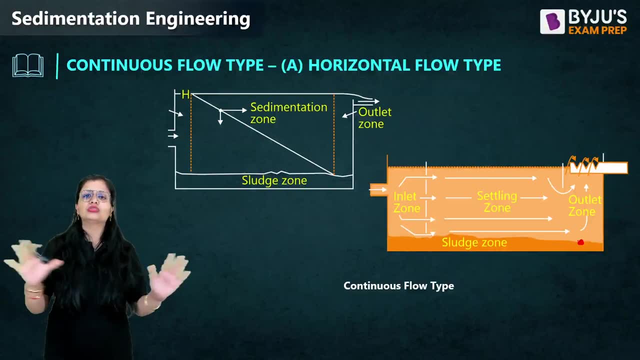 are taken to simple our calculations. So we assume that if a particle reaches at the bottom of the settling zone, or you can say the top of sludge zone, it is removed firstly. Secondly, we also take an assumption- see, obviously different size of particles will be there. obviously it's not like only 5 mm size. 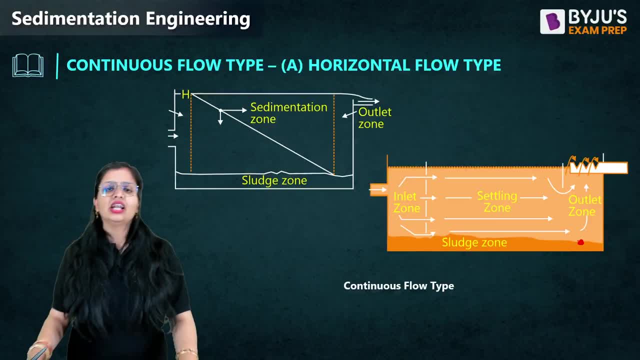 of particle will be there or 4 mm size of particle will be there. the concentration, the type, the size of particle varies Eventually. we take it as spherical, that is an assumption. but we assume that the particle is the concentration of particles because obviously size will vary. for 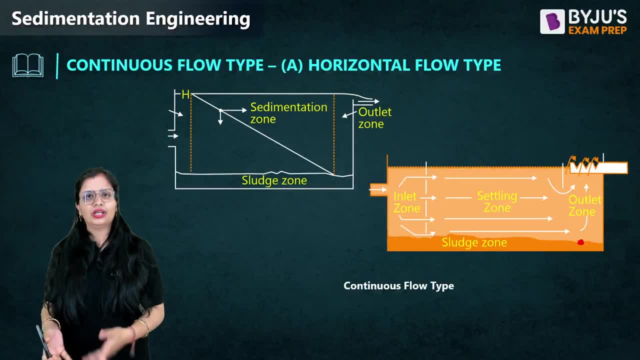 sure it's not. you'll get 2 mm particles throughout the time, only no other size. it's not practically feasible and practically possible. So generally, what happens we assume first is a particle is said to be removed if it reaches the bottom of the settling zone, or you can say top of 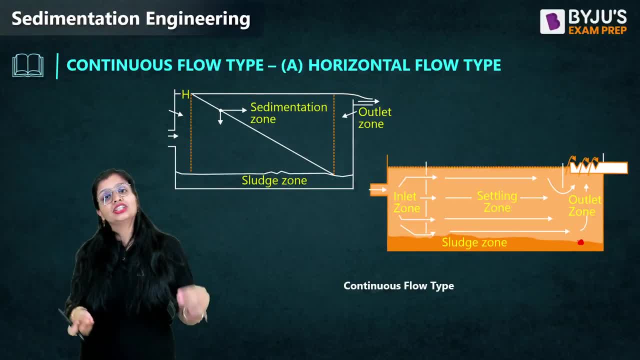 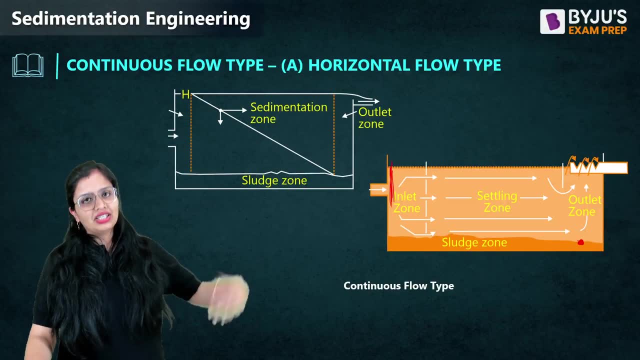 sludge zone. Secondly thing comes: concentration of particles. So we assume that the particle is the concentration of particles, because obviously all the particles, all the sizes across the vertical section of the inlet end, okay, we assume it is the same. So if 5 mg per liter of a particle is there, okay, this is the concentration of. let us 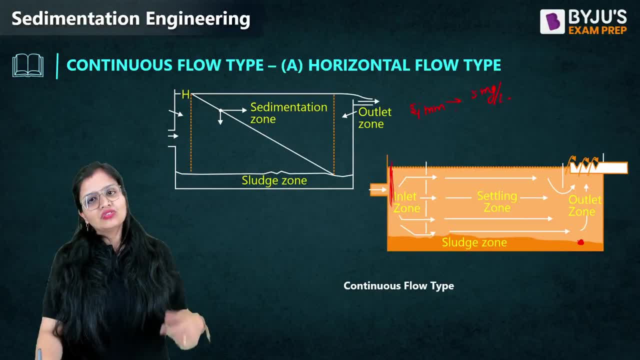 suppose 4 mm size of particle. So we'll assume this 5 mg per liter particle. and let us suppose the size of the tank. example I'm taking arbitrary: 10 meter is the height of the tank. So we'll assume per meter you will be getting what? per meter you will be getting the same concentration. 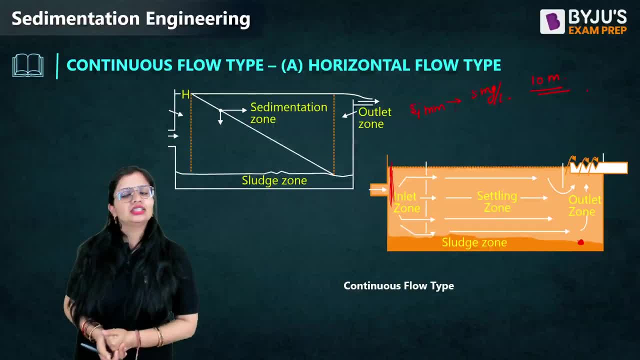 of particles along the vertical section. This is the meaning of it. Okay now, but the question is not answered. ma'am, The turbulence is not zero. how will the particle be removed? So, eventually, what will happen? when the particle is traveling forward, it is also traveling downward. 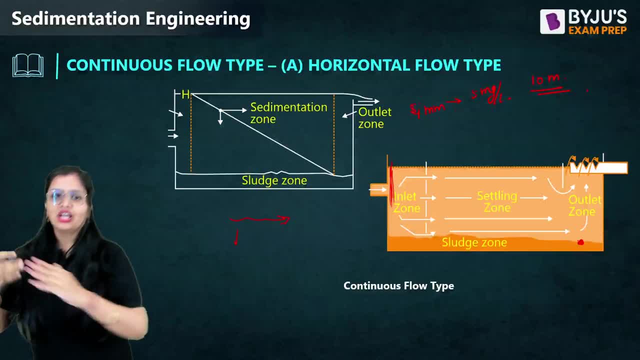 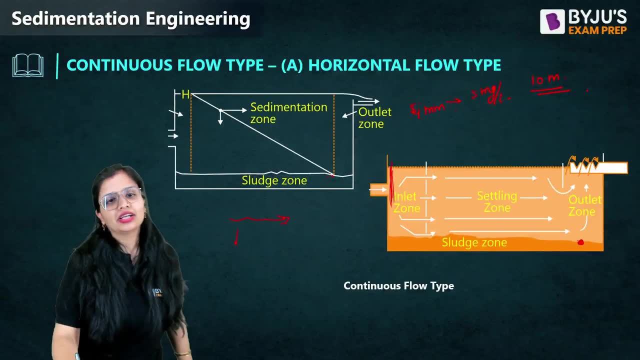 So it is traveling forward, downward, forward, downward. So what is happening? forward, downward? So, eventually, till the end of the tank, when it travels that l length, eventually the particle was here, will go here. Okay, So along with the flow velocity in the forward direction, it has a settling velocity. 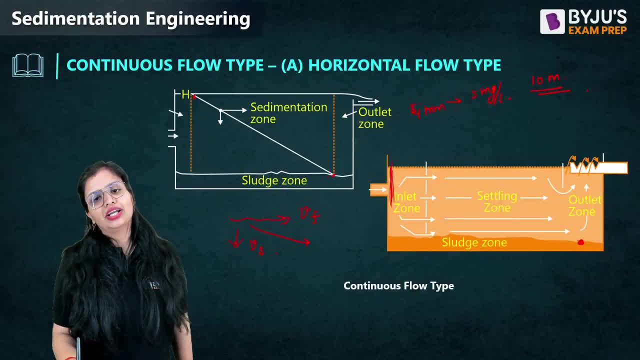 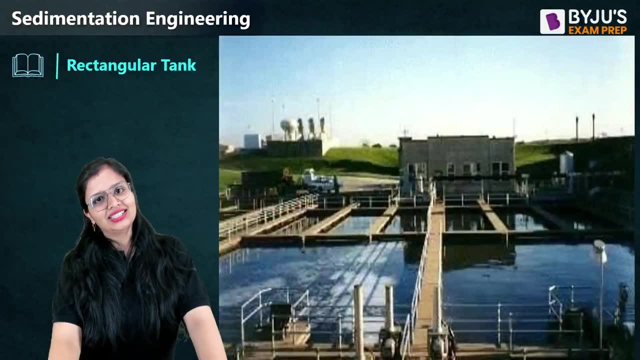 in the vertically downward direction. That is the resultant which you are getting here Clear. So this actually takes place. So you are not making the turbulence zero in this case. Now you can see one of the rectangular. generally it's not rectangular. the plan is rectangular. 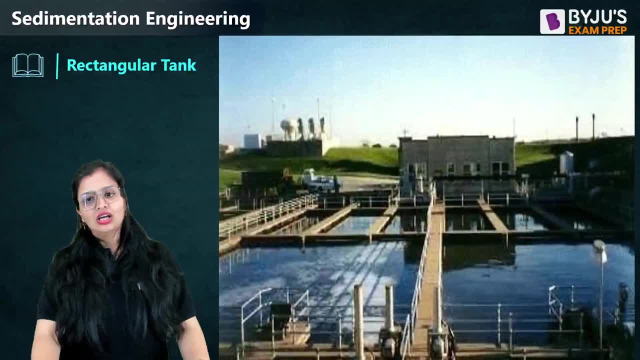 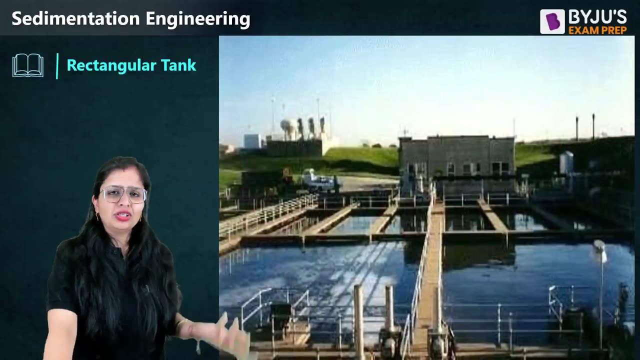 Okay, when you see it from the top, you will see it as rectangular, So you guys can see the the pixel. Actually, I take it from Google, So the pixels are not that proper, but you'll get an idea how the sedimentation tank basically looks like. Okay, If it's possible, you guys can go to the. 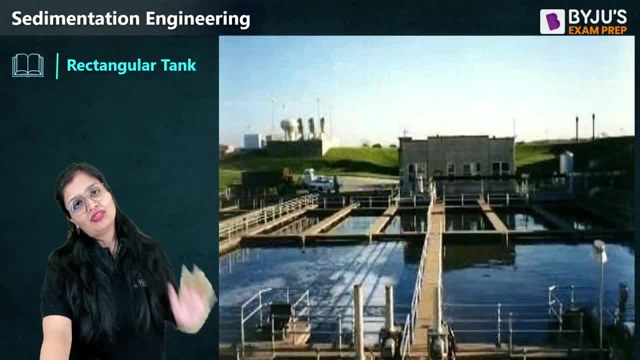 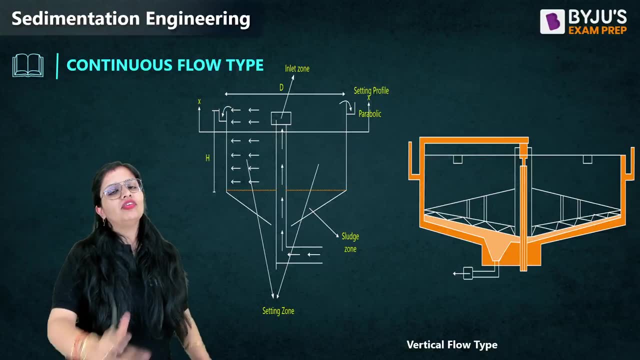 nearest treatment units in your cities and you can have a look at it. Okay, Now you have rectangular. similarly, you have what vertical flow type tank? You have horizontal flow type tank. Similarly, you have vertical flow type tank. Now you will be like ma'am, what is the difference between that? 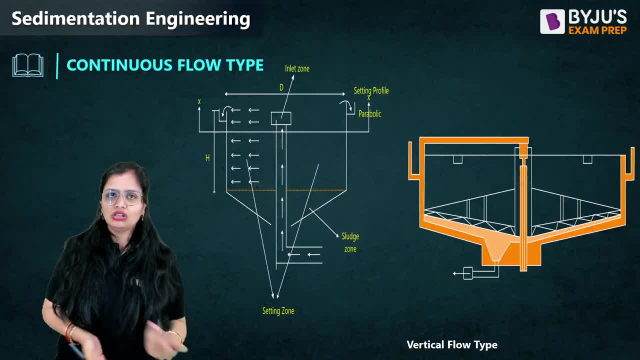 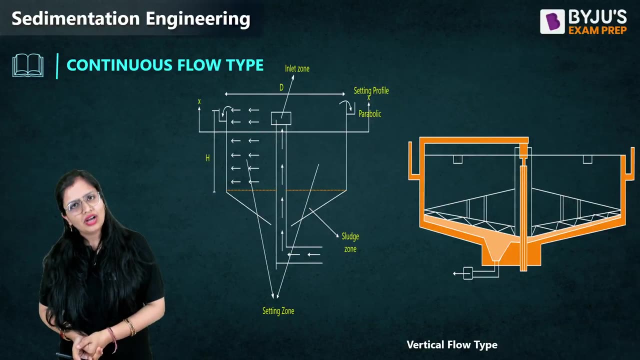 See, When you were talking about rectangular horizontal flow type tank, in that you were talking about the rectangular plan was there The resultant velocity was linear. But here the resultant velocity is not linear, It will be parallel. Why Why? Because here the movement of water. you can see that there is a central pipe. 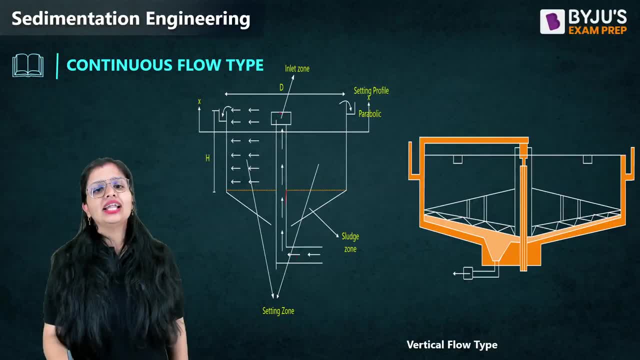 A central pipe is there from which the water moves, and then the water moves like this, on both the sides, on both the sides. Eventually, the suspended solids will settle and you can see, if you want to see here, the suspended solids will settle and it will be removed through proper mechanism. 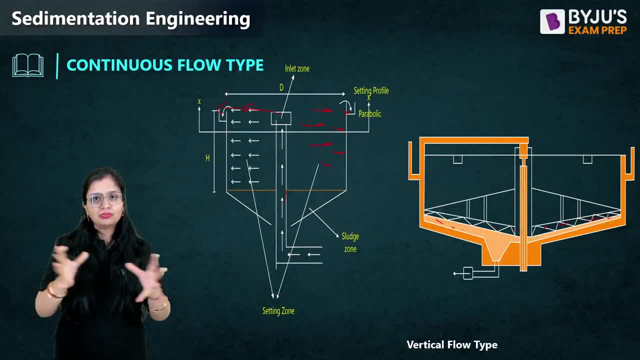 So here the flow of water takes place radially. You are not dating the resultant velocity as linear, which you used to get in the case of horizontal flow type tank. Okay, Generally the plan of it, If you talk about it, is circular in nature and if you have difficulty in visualizing 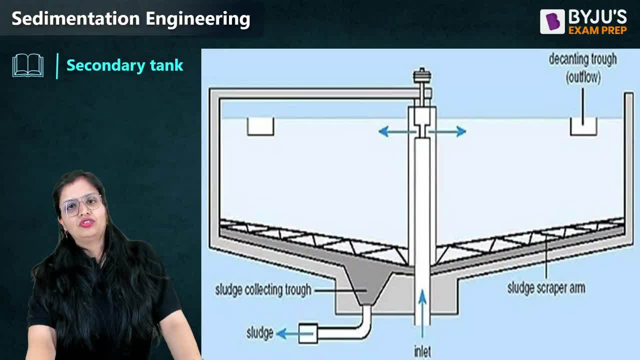 you can go through this. This is just the figure which I have told you. This is the only figure. This one is the only figure which I have told you here. Okay, But I have broadened it. You see, water will move in radial direction. 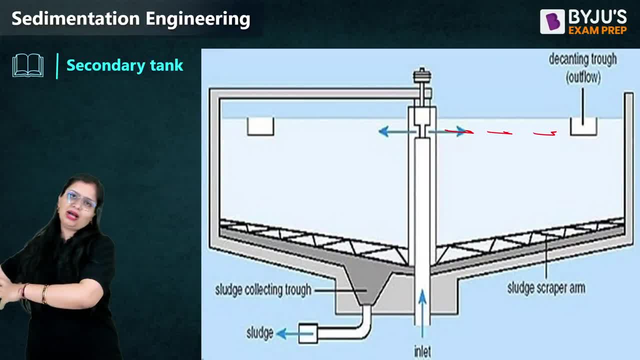 Water will move in radial direction, It will be collected and it will be passed further, whether it is for filtration or any other process. Why The sludge will be collected from bottom? because obviously the fine Suspended solids will settle under its own weight. and what will happen? formation of 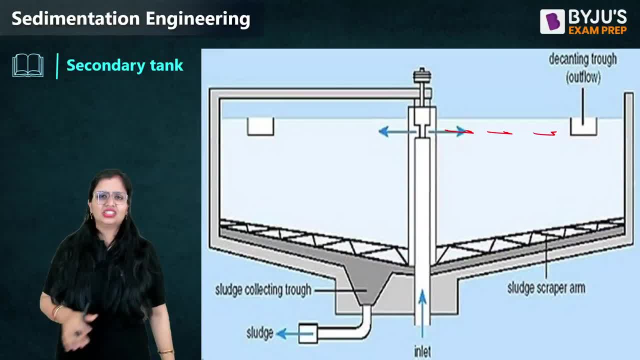 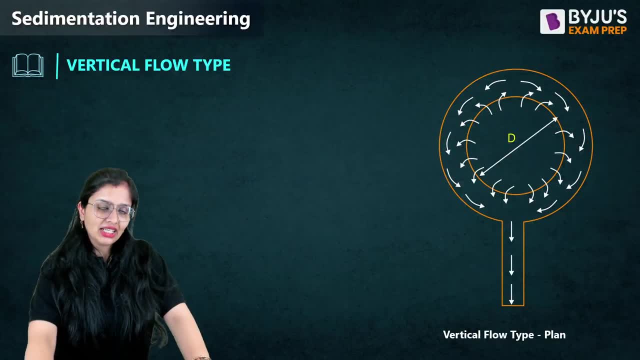 sludge will take place and, depending upon whether the organic concentration is there or what not, they will be dispersed. Okay, Now talking about next is if you talk about the plan. Plan is when you look at from the top, you will see that the plan is circular in nature. 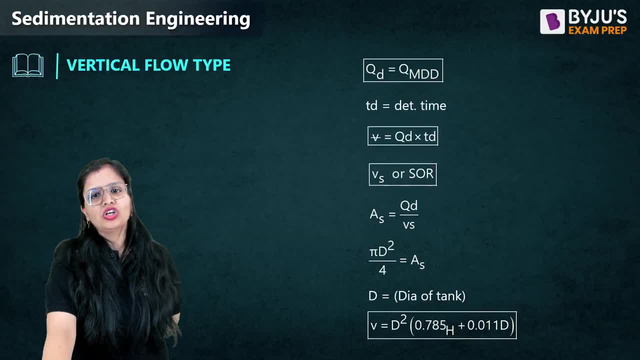 and you are like you want to calculate the volume. So the volume is given empirically. How, If you talk about volume is given by d square 0.7855.. H plus 0.011 T. This is very much prevalent. 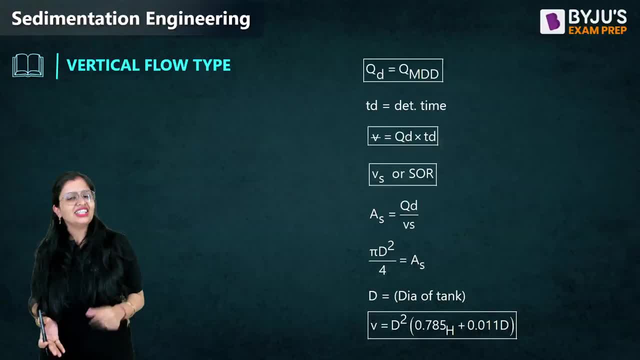 Here also: you design it for maximum daily demand. The detention time is comparatively less. It varies from whether it is 2 to 6 hours, whether it is for plain sedimentation or you are adding some chemicals. If you are adding some chemicals, the detention time reduces. 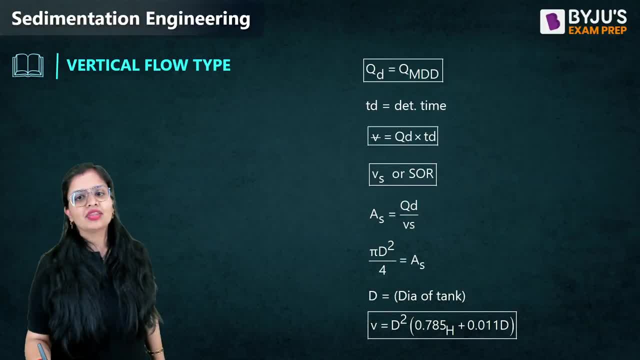 Okay, Volume is equal to discharge into detention time, which has been mentioned to you: Settling velocity. Settling velocity is the velocity, The velocity with which the particle settles in the tank, or you can call it as the surface overflow rate. 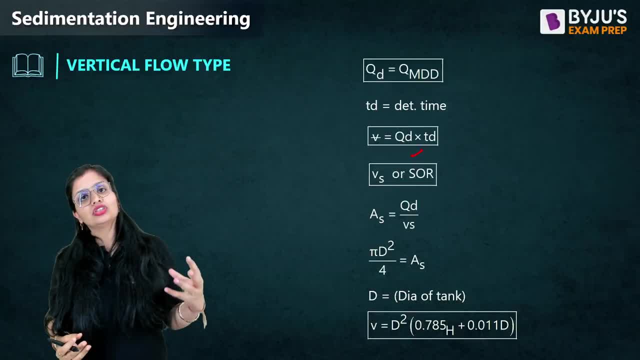 Okay, Surface overflow rate. Let me tell you this is the velocity of the design size of particle. Let us suppose when you are designing a tank, you design it for a certain amount of discharge. Similarly, you design it for a particular particle also. 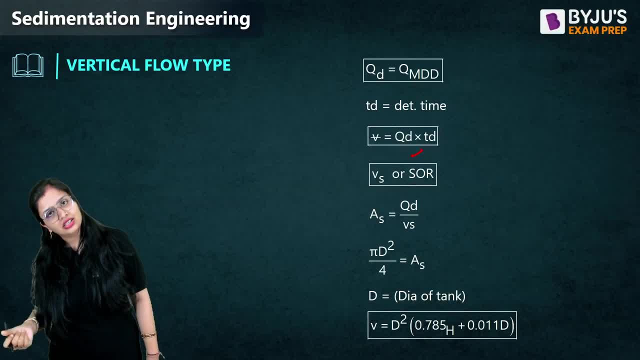 Okay, So the velocity of that concerned particle is known as surface overflow rate, or you call it as velocity of the concerned size of particle. So if you talk about Settling velocity, VS or surface overflow rate, in short, you call it as SOR. 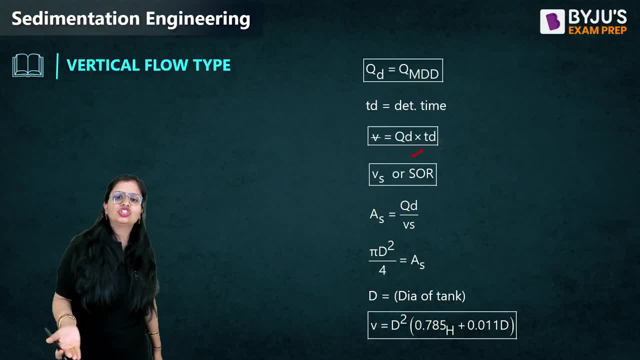 Okay, So if you want to calculate area, area is equal to discharge upon velocity and area. if you look at the plank of the vertical prototype tank, it is circular, So area will be pi by 4D square, with the help of which you will be able to calculate. 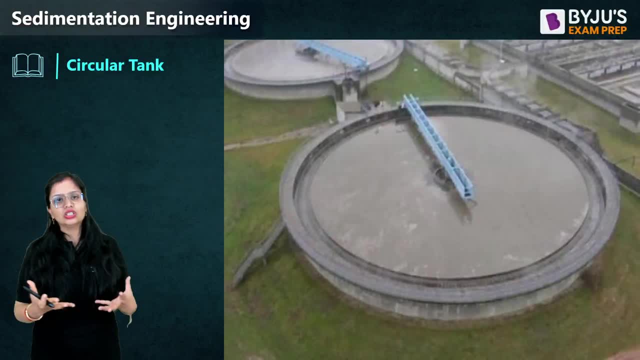 that diagram And if you want to visualize how the circular tank looks like, So you can see, this is the circular sedimentation tank. Here also, The movement will be taking place, the turbulence will not be zero and what you will see is here. 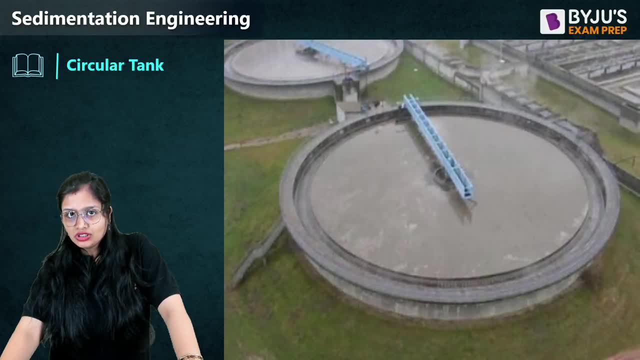 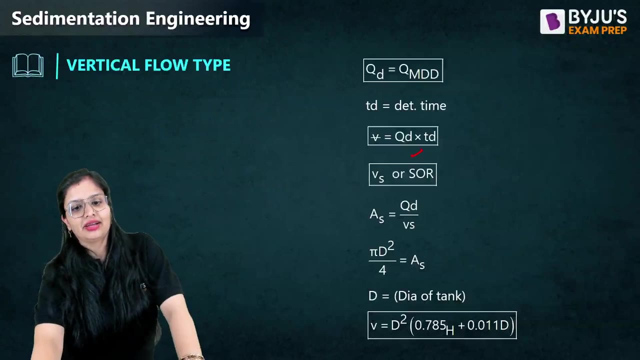 during the movement. the resultant velocity will not be linear, it will be parabolic in nature, and you will see here that the sludge will be collected at the bottom, which will be further taken out. Okay, So this is regarding circular sedimentation tank. 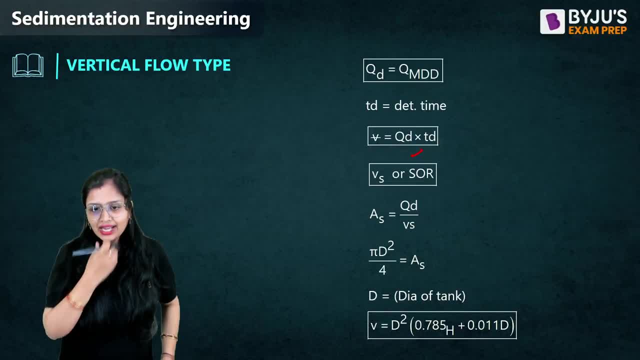 One more thing I told you regarding vertical flow type tank. Now here is one more thing. So this is circular sedimentation tank. One more thing is there, if you want to calculate the settling velocity of the particles, because I just told you, Vs is the settling velocity or the surface over flow rate. 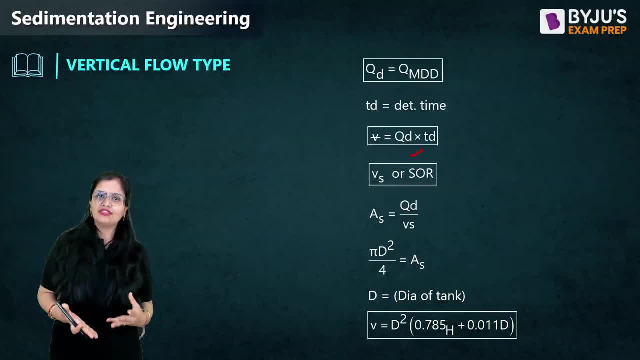 Now how to calculate settling velocity. that is given by Stokes law when you assume that the particle is spherical in nature and all those things. So if you want to calculate settling velocity, there are different things. Different things means whether the flow is laminar, whether the flow is turbulent, whether